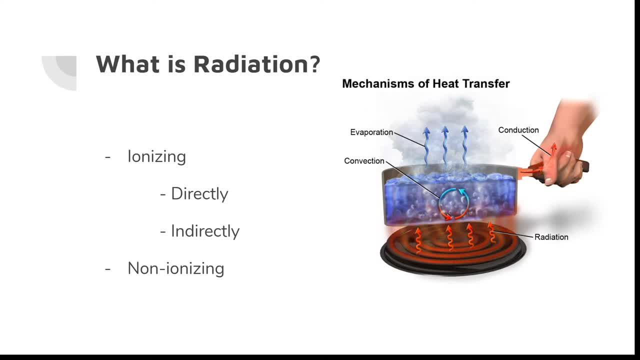 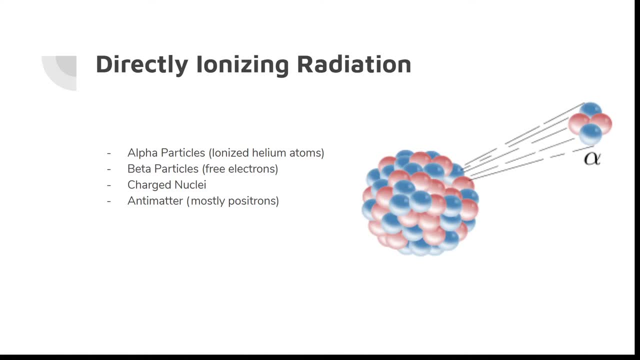 This is opposed to non-ionizing radiation, which doesn't tend to affect materials. Ionizing radiation can also be broken down into two groups. The first group, called directly ionizing radiation, includes alpha particles, beta particles, charged nuclei and antimatter. 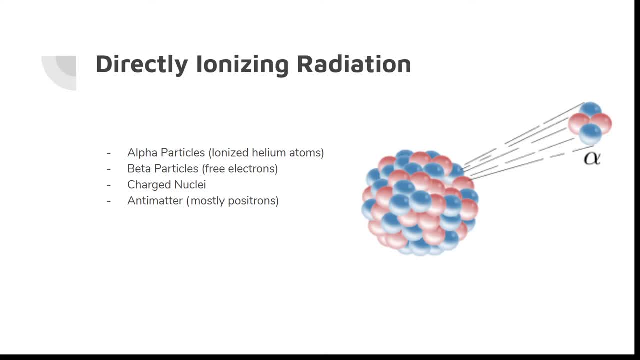 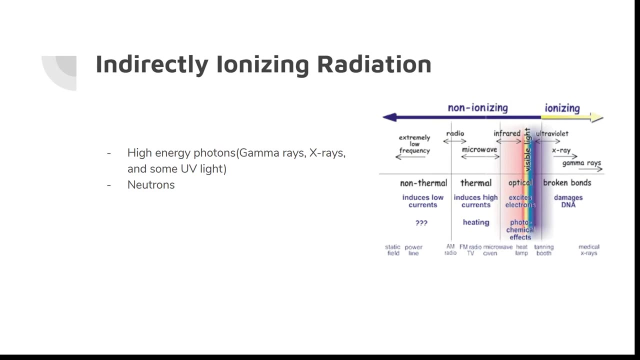 Most commonly in the form of positrons. Directly ionizing radiation, as the name implies, directly causes an ionization event when interacting with an atom. The second group, called directly ionizing radiation, is called directly ionizing radiation. The third group, called indirectly ionizing radiation, includes high-energy photons, gamma rays, x-rays and, in some cases, UV light and neutrons. 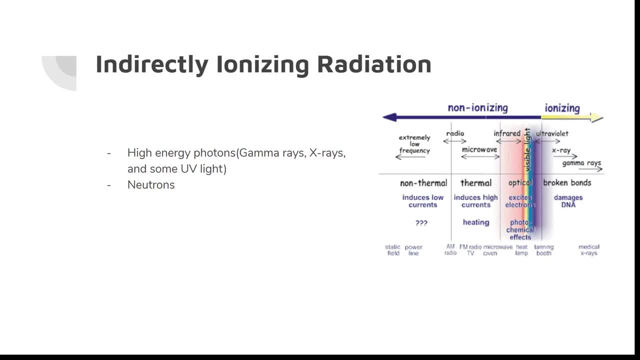 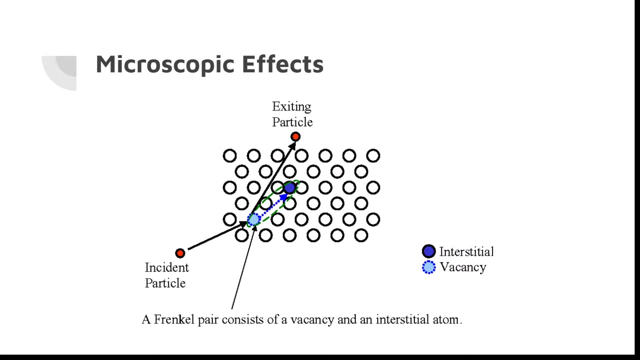 Indirectly ionizing radiation doesn't immediately cause an ionization effect upon interaction with an atom. Instead, the resulting interaction results in directly ionizing radiation, which will then ionize a different atom. So now if we think about incoming radiation, 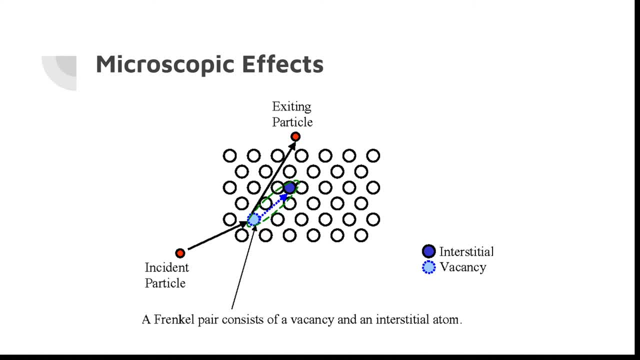 If we think about incoming ionizing radiation with some kinetic energy interacting with a material, it seems kind of obvious that it would interact with an atom of the material, making that atom ionize and giving it kinetic energy. This atom would move around the material, leaving a vacancy where it started. 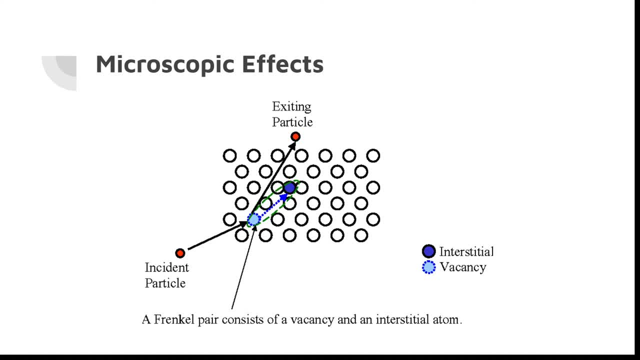 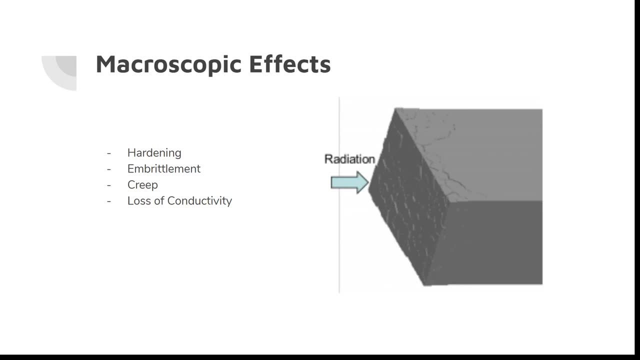 and potentially have a similar effect to other atoms it interacts with until it finally stops as an interstitial atom. This increase in interstitials interaction, The material's macroscopic properties, are several ways It causes: hardening, embrittlement, irradiation creep and loss of conductivity. 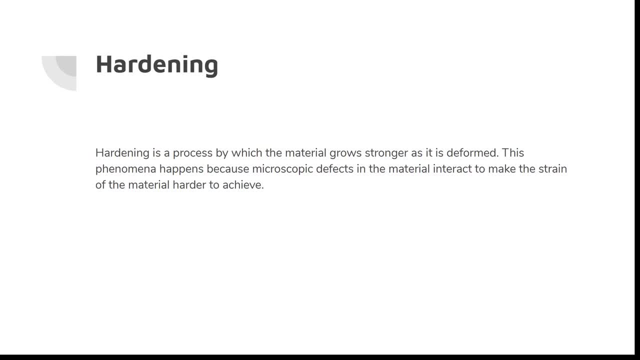 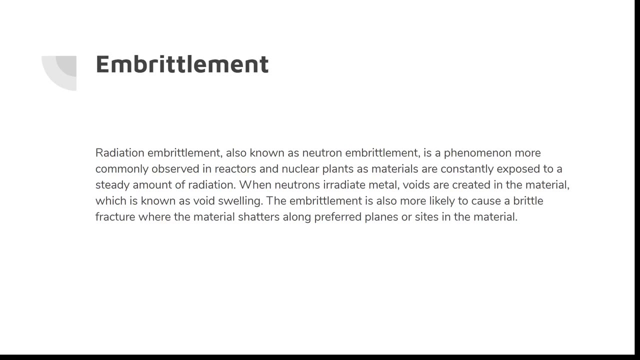 Hardening is a process by which the material grows stronger as it is deformed. This phenomenon happens because microscopic defects in the material interact to make the strain of the material harder to achieve. Radiation embrittlement, also known as neutron embrittlement, is a phenomenon more commonly observed in reactors and nuclear plants, as materials are constantly exposed to a steady amount of radiation.